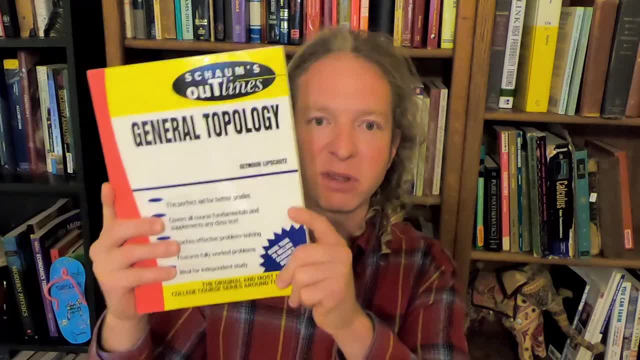 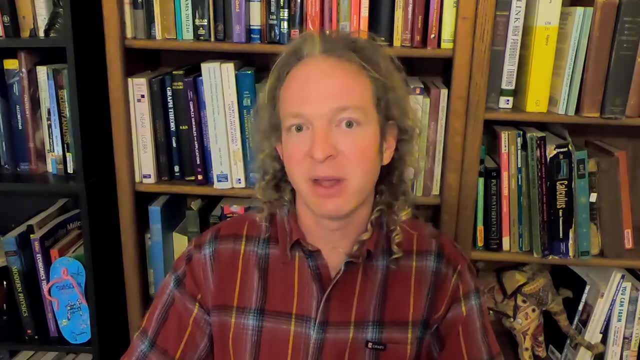 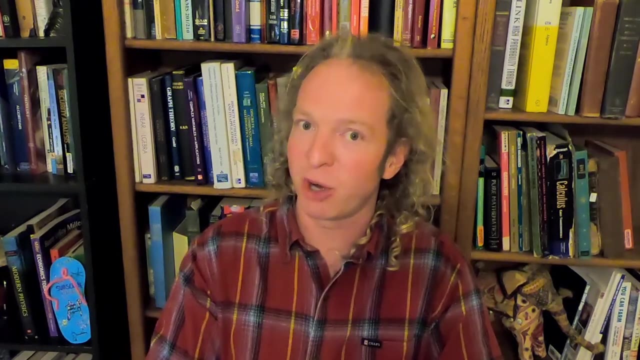 topology And, as most Shams, they are pretty good, But this one in particular is extremely good. So the Shams outline on general topology is one of the best ones. In my opinion it is the second best Shams. I think that the complex variable Shams is even better than the topology one. 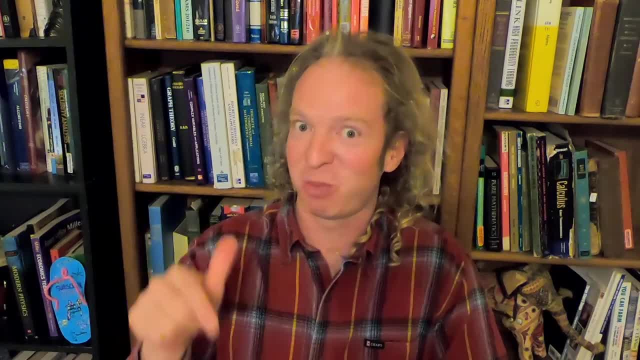 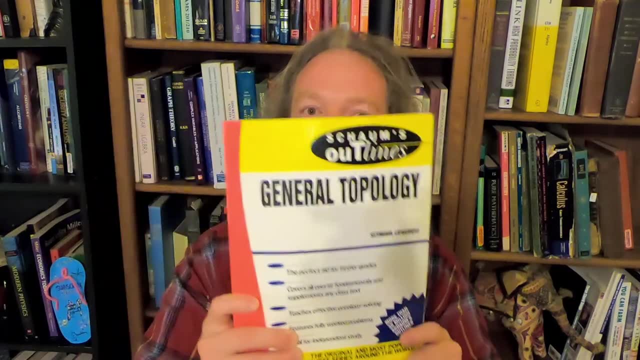 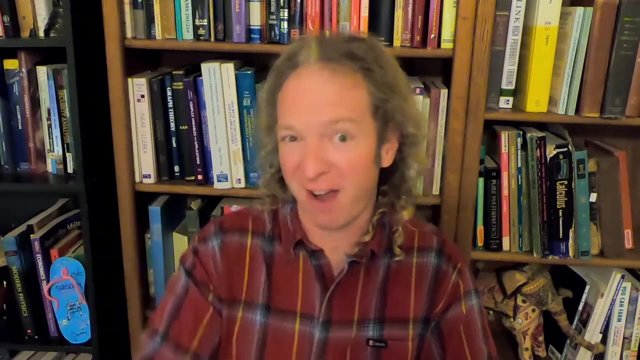 But that's not what this video is about. This video is about topology. This book is really good because it goes well with whatever course you're taking in college. So if you're taking a topology course in college, everything you learn in your course you'll find in the 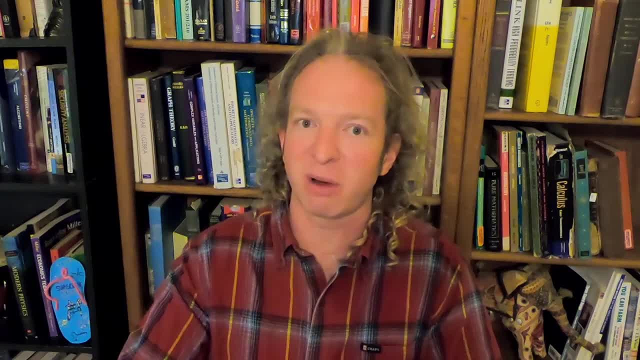 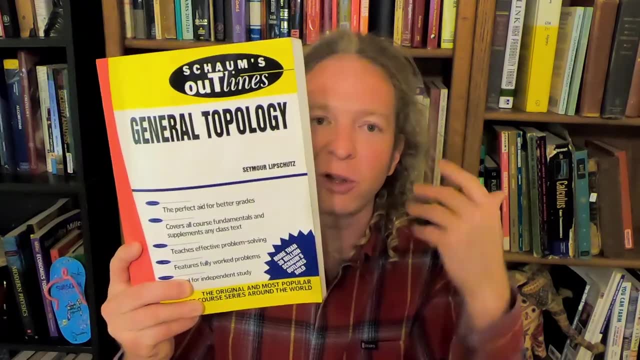 Shams book, right. Same thing with Moncrief. It's a great reference. So, if you're taking topology, they both serve as great references And this book is really easy to use. If you want to look up, hey, what's a T1 space? Just look it up. It's in here, right? It works out really, really nice. 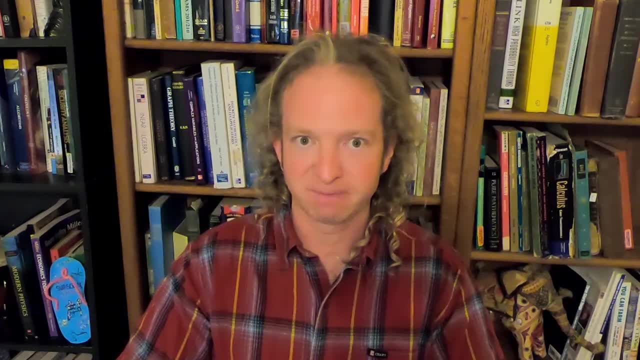 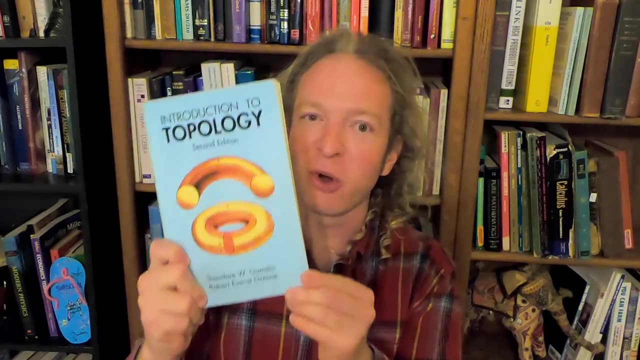 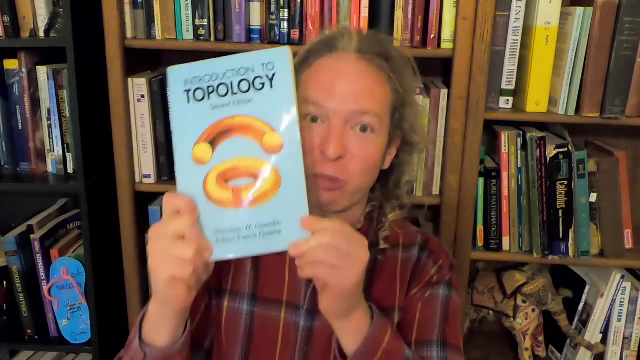 as a supplement to your course. I saved the best for last. This is topology by Gameland and Green. This is a Dover book, which means it's only a few dollars, even brand new. It's not expensive. This book has solutions to every single problem right. Every single problem in this book has a 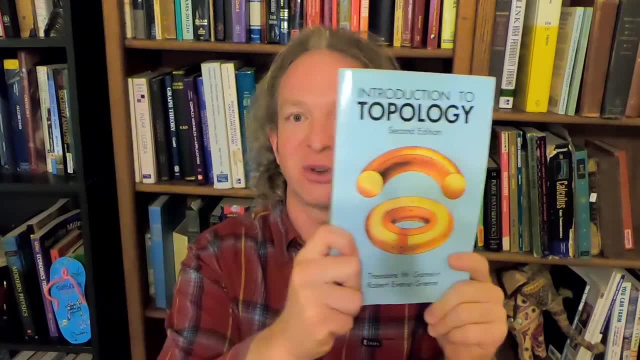 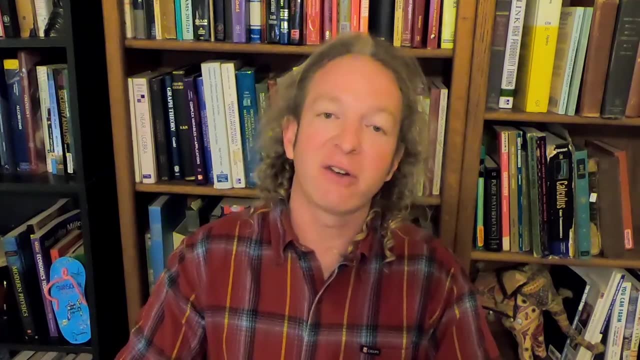 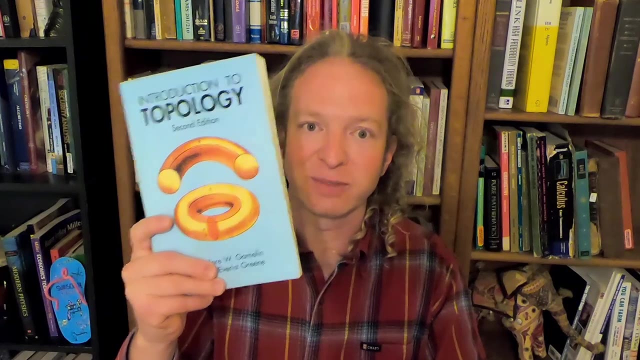 solution. The proofs have proof sketches. So again, it's topology by Gameland and Green. I have used this book for self-study, I have read portions of it and I have also done several of the problems. This is a great choice, And again for only a few dollars. So there you. 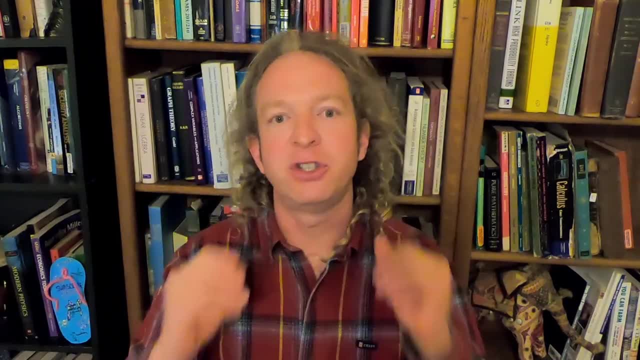 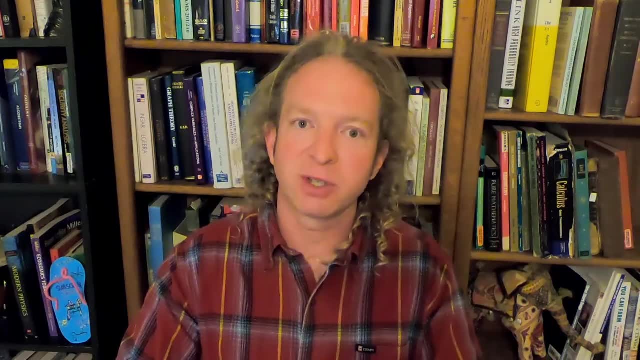 have it. Those are three choices for topology books that you can get for just a few dollars. I will leave links to the books and full book reviews for each book in the description. If you have any other suggestions on good topology books, please leave a comment in. 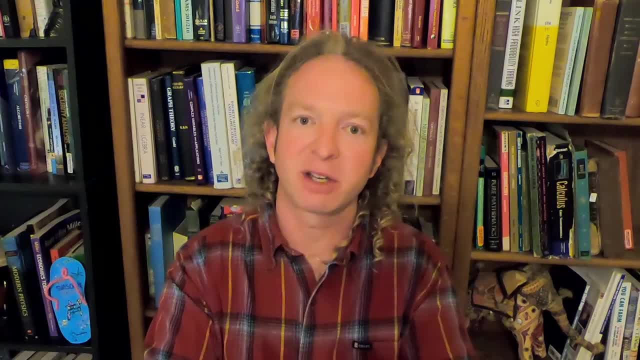 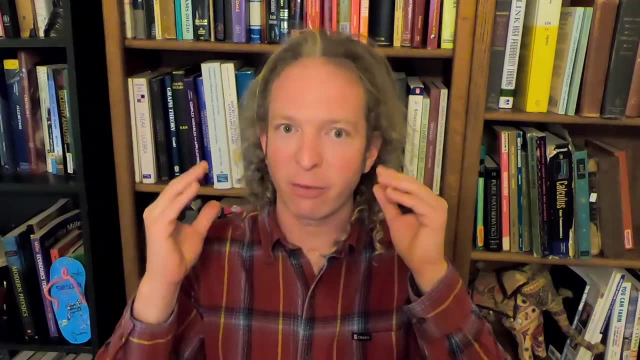 the comment section below. If you have any questions, please leave a comment in the comment section below. Again, there are many other books on topology. I just wanted to talk about three, So you can go out right now and if you want to pick up three books, that are good. 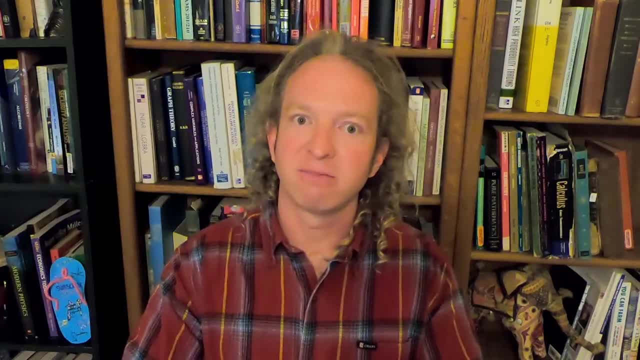 that are good, solid topology books. you can do that now. That's it.